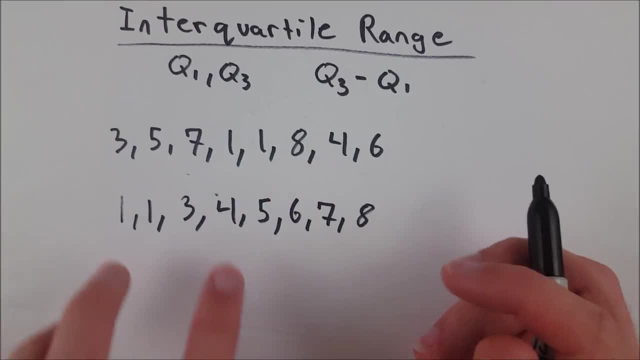 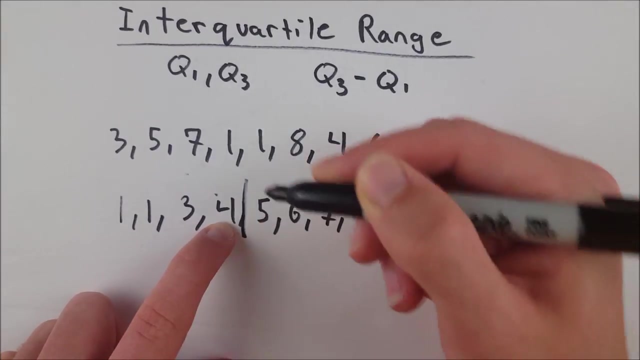 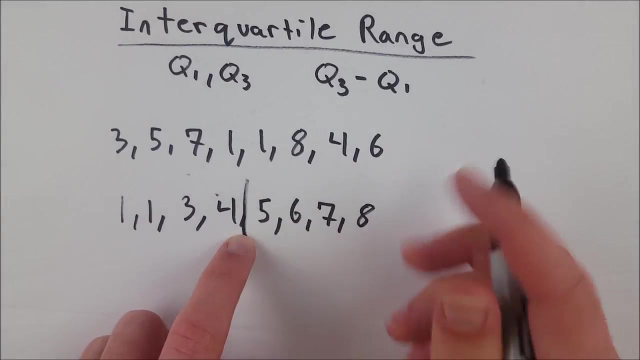 Now we want to split the data basically in half, So we have 50 percent to the left of our split and 50 percent to the right of our split. We're going to do this basically by finding the median. So you can find the median of a small set of data, you know, just by counting in from the end points. So you go in one, two, three and then you see we've got two numbers here in the middle. So we'll put our split between the two numbers in the middle. If we had an odd number of data- Let's say we had another four here- we would just split the data there. So we'd have these numbers down here and these numbers up here, and then this four would just the extra four that we're pretending would be here. We would just 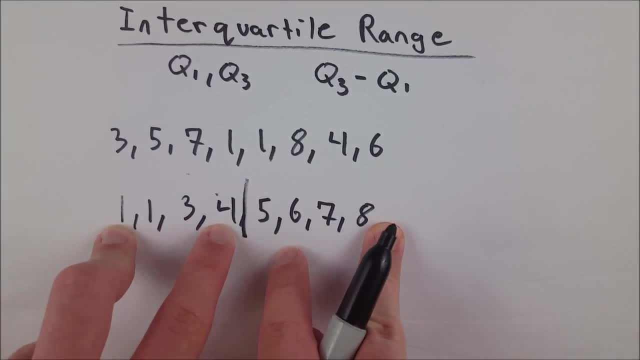 and we're only going to be concerned with these two halves of the data for finding the interquartile range. So now to find the first quartile, of course we just need to find the median of this lower half of data. Go in 1,, go in 2, the 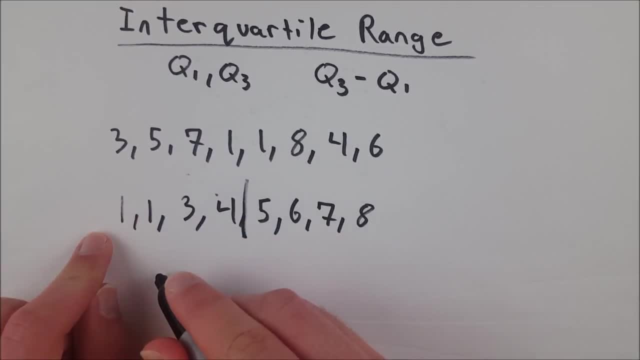 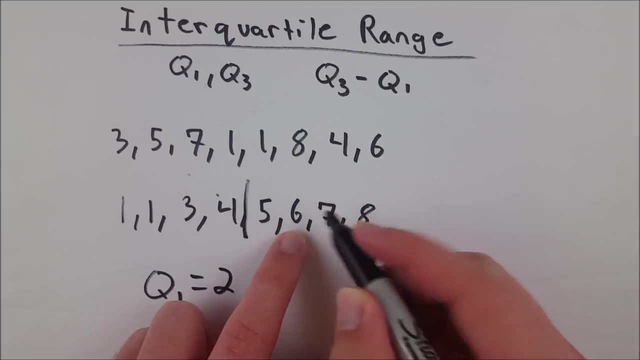 median of this lower half of data is halfway between 1 and 3, so it's 2.. That's the first quartile, And then, over here, go in 1, go in 2, the third quartile is halfway between 6 and 7, because that's the median of the upper half of data. 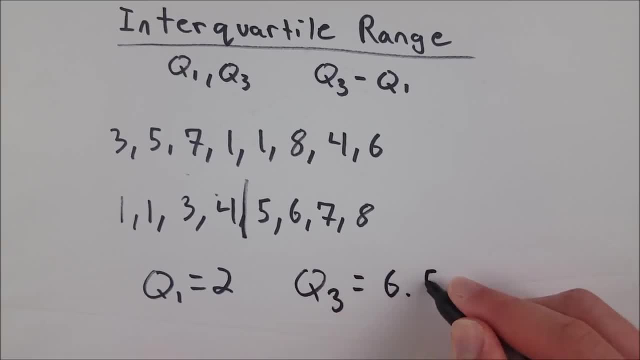 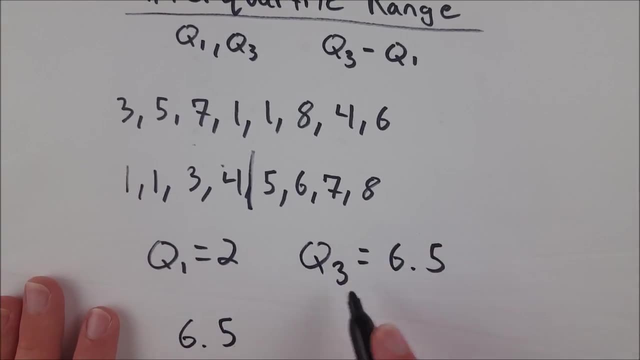 So the third quartile is equal to 6.5.. So the interquartile range is 6.5.. Whoops, let me slide this up a little bit. That's the third quartile minus 2, the first quartile, as you can see, and that's equal to 4.5.. So our interquartile range: 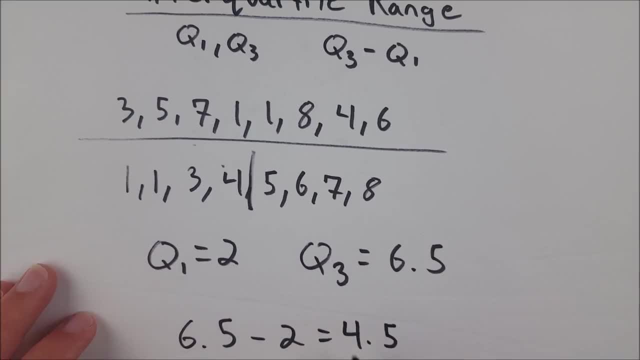 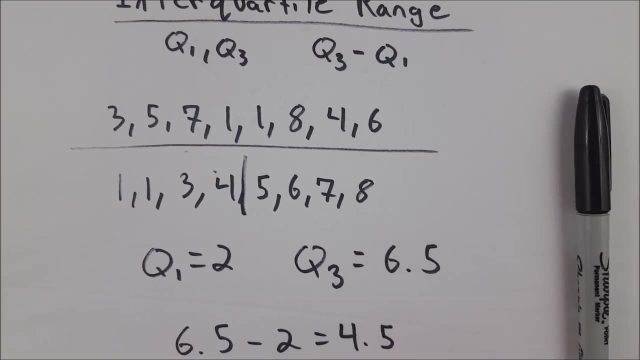 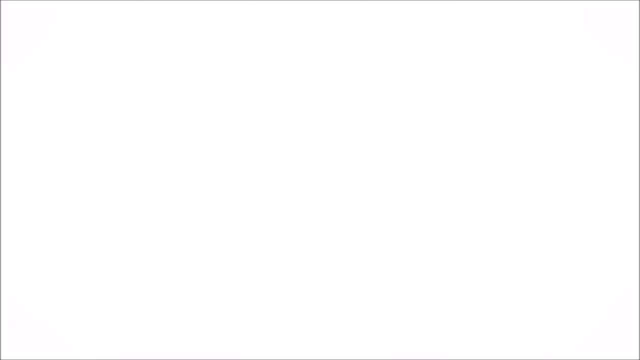 enjoyed this video. I hope it helped you understand how to find the interquartile range and, of course, how to find the first and third quartiles of a set of data. Let me know in the comments if you have any questions, if you need. 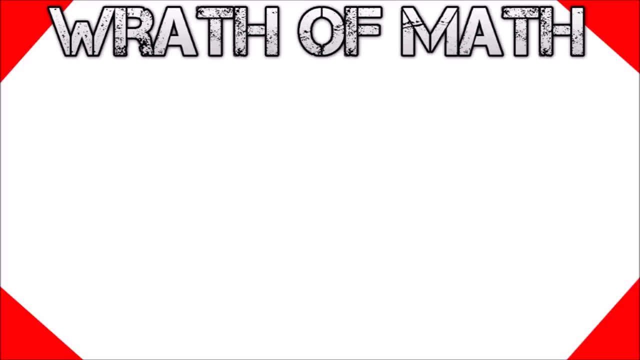 anything clarified or have any other video requests? I'll see you next time. Thank you very much for watching and be sure to subscribe for the swankiest math videos on the Internet.